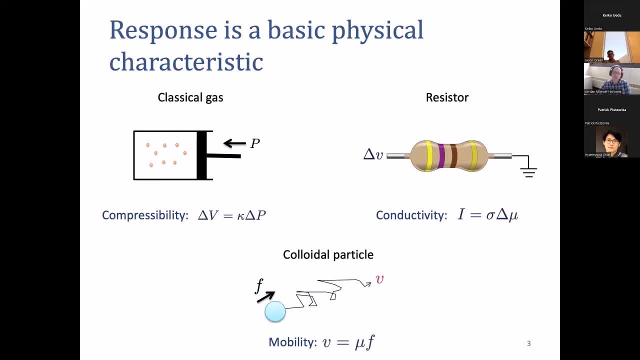 a lot of different sources but the names are always different, so it's kind of hard to kind of rationalize everything. And maybe a classic example would be a gas where you increase the pressure on the gas and look at the volume change, The response property, the response coefficient. here 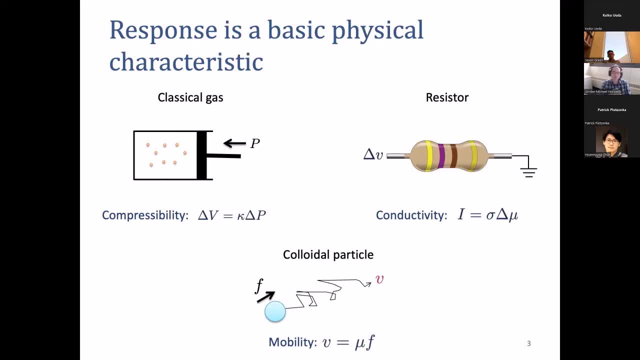 is the isothermal compressibility and characterizing. that is important because it tells us about the density of the gas and the strength of inter-particle interactions and the like. Another nice example is maybe a resistor, where you want to characterize it by, say, applying a potential difference across. 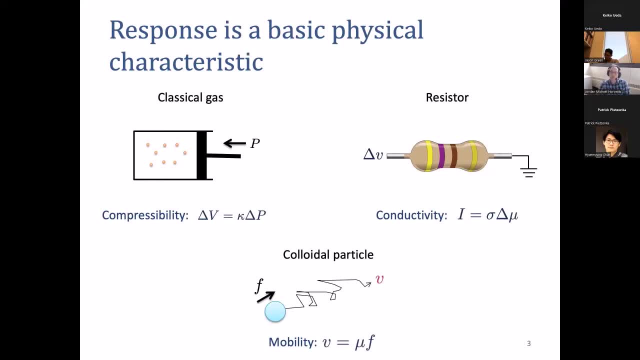 the resistor, So the current is generated. Of course, the proportionality constant of the response function here is the conductivity, And the knowledge of the conductivity tells you things about the electronic properties of the resistor. It's also very important say for applications: where you want. 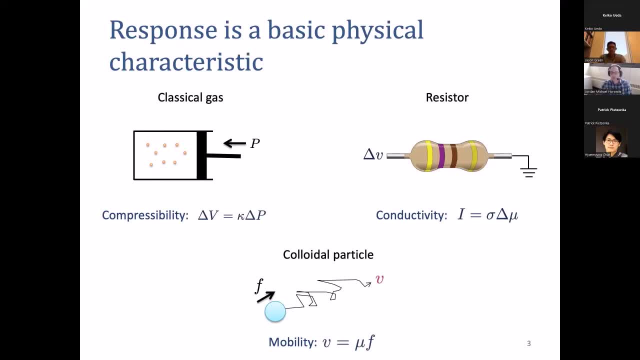 to know these properties so you can engineer them and put them in the right place in your physical system of interest. Another classic example is: say, maybe a colloidal particle immersed in a viscous fluid. You apply an external force, you're going to generate some velocity. 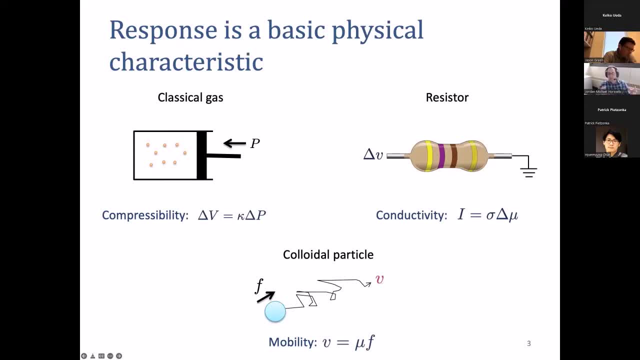 The proportionality constant here is the mobility and of course it tells you about the size and shape of the particle and properties of the background fluid like its viscosity. So despite all the different pictures here, they can all be kind of rationalized or 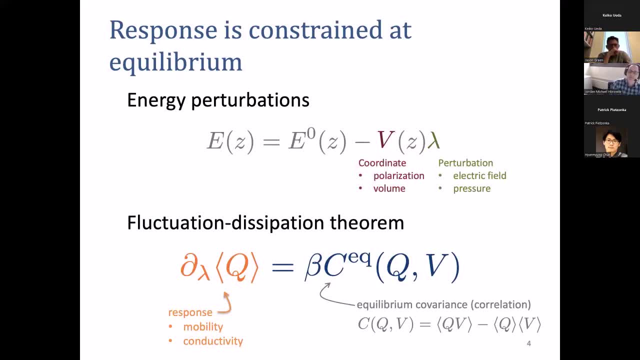 understood or unified within the context of linear response theory. And a very general setup here is: we have some physical phase space variable, state space variable and some unperturbed energy, And then we apply some external perturbation. We turn on some external field which I'll call lambda. So the lambda could be an electric field or apply a pressure. 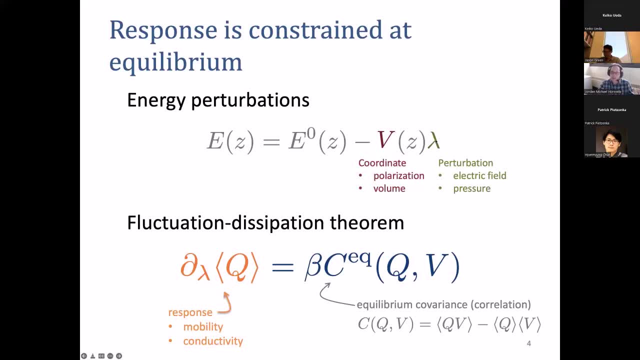 And then when we change this parameter, we're going to do work on the system and change the energy, and the amount of work depends on the product of lambda and its conjugate coordinate right. So this is the work. So, for example, the electric field is conjugate to the polarization. 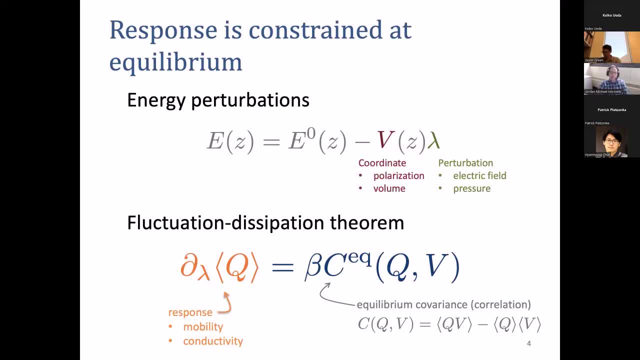 or the pressure is conjugate to the volume. And now the kind of central prediction of linear response theory is the fluctuation-dissipation theorem which tells us if we look at the expectation of some observable, its response or the derivative of the expected external parameter. 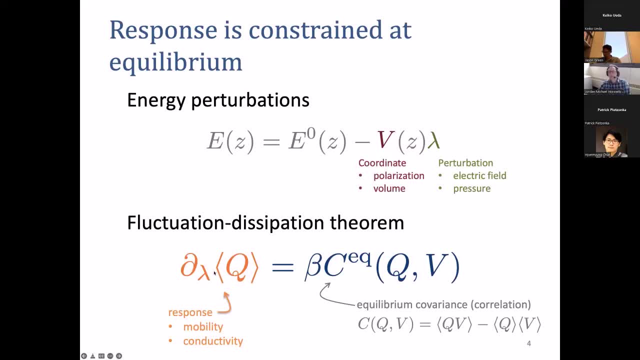 these are the material coefficients we're interested in. we're interested in the block specifications. we're interested in the energy distribution. we're interested in the energy we're interested in, like mobility or conductivity, that we can always write this response as proportional to the equilibrium correlation function. 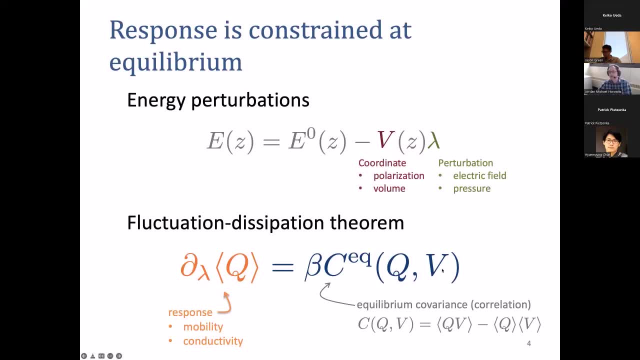 between the observable of interest Q and some conjugate coordinate V that appears in the energy. And this is useful for two basic reasons. One is we always know the proportionality: constant, it's universal and system independent, it's the inverse temperature. 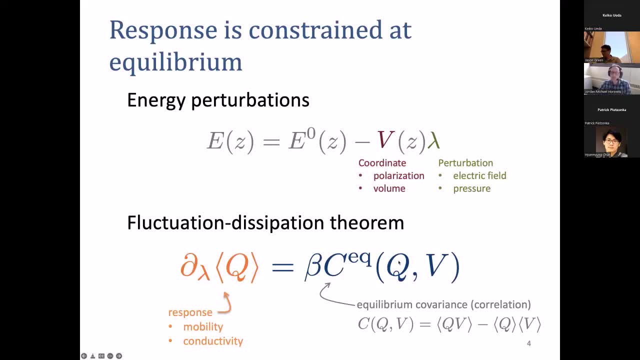 And we have a pretty good understanding of, say, mechanics and equilibrium statistical physics, so we can extract what is the appropriate conjugate coordinate. One really interesting application of the fluctuation dissipation theorem is that if I don't have to actually do the response experiment, 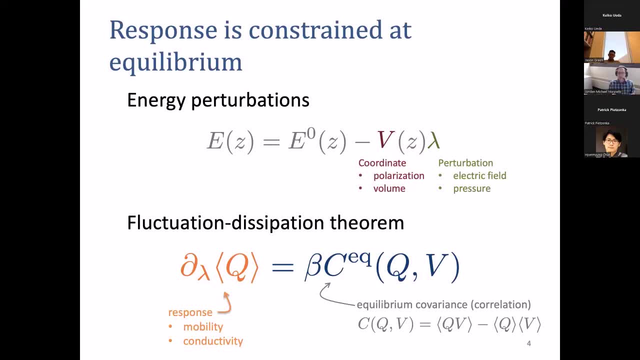 I don't actually have to kick the system, I can just sit back and watch the fluctuations and extract the same information right. So that's the kind of basic idea that underpins something like micro-rheology, Another application which is perhaps somewhat little less appreciated. 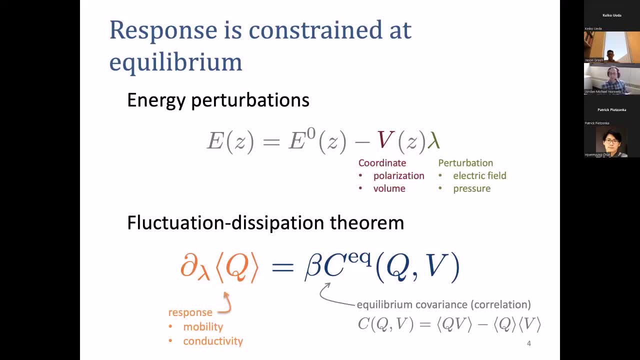 is that if I wanna build a really sensitive device like a measurement device that amplifies my signal a lot, if I build that at equilibrium, I will necessarily have a lot of noise right. So when I make a very good measurement device that's very sensitive. 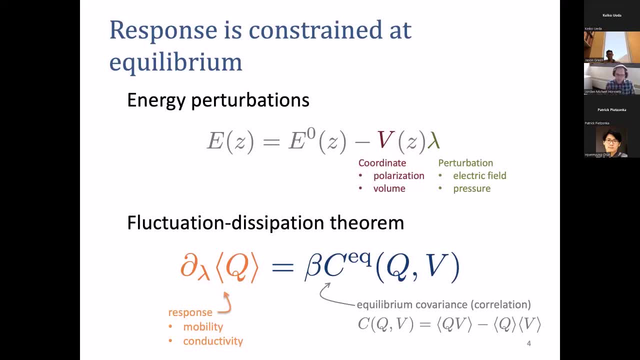 it will also be very noisy, which is bad. So if I wanna do better than that, I have to go out, I have to break detailed balance, go out of equilibrium and burn energy. So this kind of sets the stage of where we wanna go. 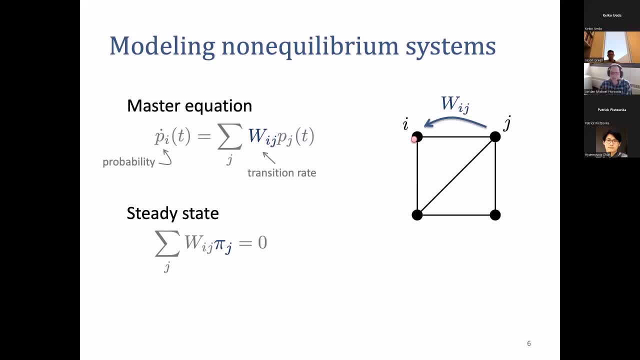 And we wanna start asking now what happens when we do break add energy, break detailed balance. How much? what can we get? How sensitive a system can we get? And at this point I need to be a bit more specific about how we actually model a non-equilibrium system. 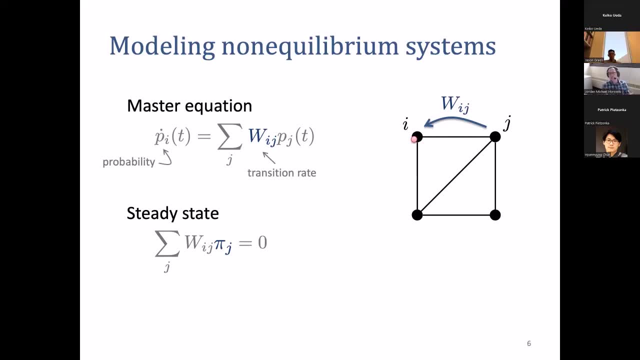 And so I'm gonna imagine a scenario where I can model my system as a discrete state Markov jump process. So I have a collection of states, I'll label I and J, I can visualize them as nodes on a graph And the system is then imagined to jump around. 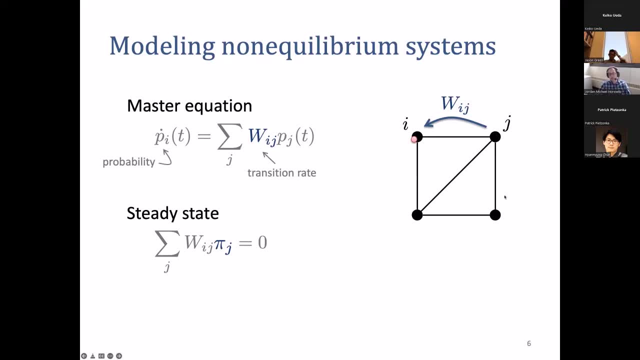 these different nodes along different edges in the graph, And the edges are the allowed transitions. So in this context, the quantity of interest is the probability to be in state I at time T And it evolves according to the master equation with a rate of change. 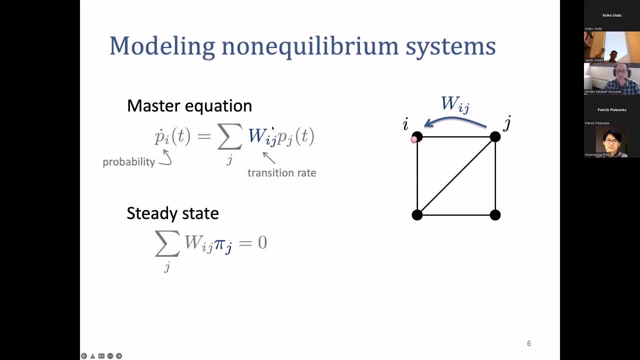 depends on these transition rates, the probability per unit time to jump from state J to state I. I'm further gonna assume, and if I don't affect the system, if I don't touch it, it will relax into some sort of steady state. 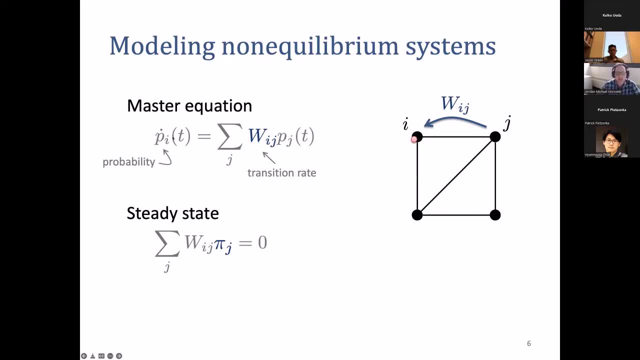 equilibrium or non-equilibrium, but it's the steady state is given as the time independent solution of the master equation, And I'm gonna label that steady state with pi. So that's just basically a model, a mathematical model, but we gotta put some physics in, right. 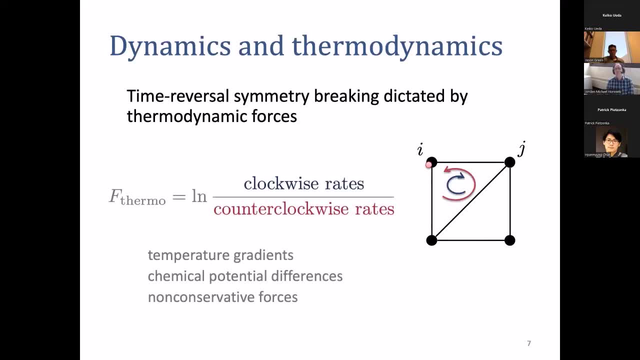 What we understand. And so in a stochastic thermodynamics conference I'm gonna assume local detail balance, And so I'm gonna recognize that if I drive my system out of equilibrium that's gonna break time reversal symmetry And I can quantify that time reversal symmetry breaking. 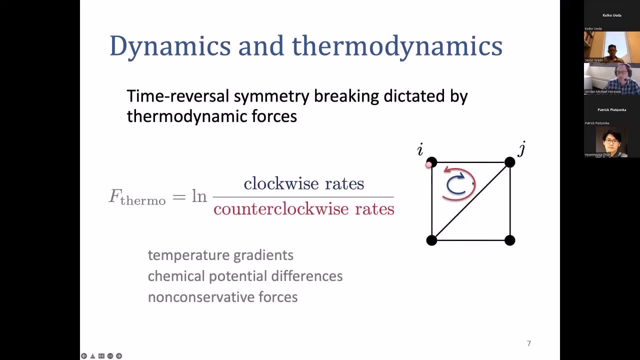 by looking at the product of rates around any cycle and its reverse. In fact, I'll look, I'll define a quantity, I'll call the thermodynamic force that measures that strength, as the log of the ratio of product rates around any clockwise cycle to its reverse right. 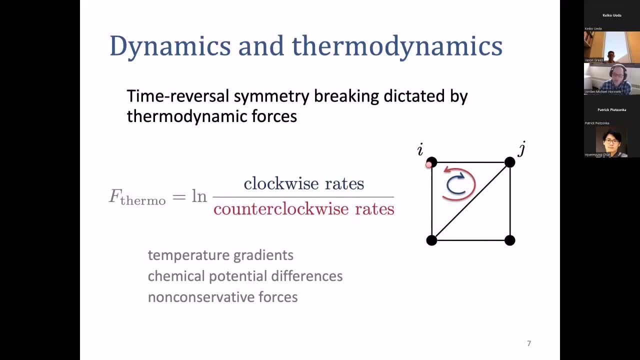 So the idea being here that if I break time reversal symmetry stronger, in principle, these quantities need to be bigger and I'll be farther from equilibrium. And if all these quantities are zero, then I'll be at equilibrium because the dynamics will be time reversal symmetric. 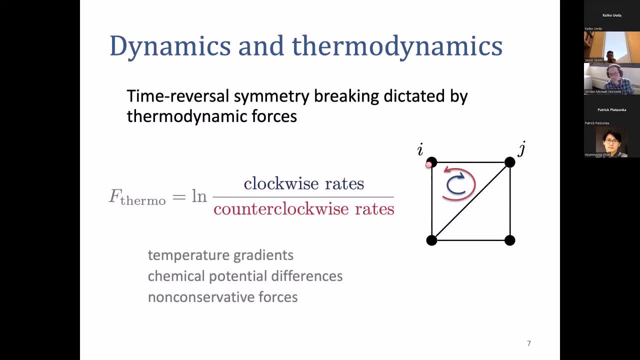 But apart from that kind of mathematical idea or ansatz, when we actually build physical models, what we do find out is that these thermodynamic forces are the kind of macroscopic control parameters that we have, like temperature gradients, chemical potential differences, non-conservative forces, 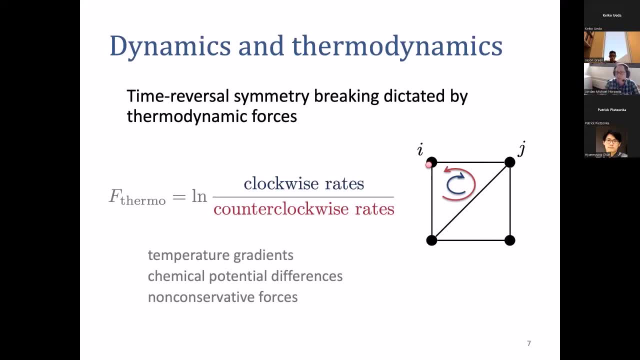 So these are things that in an experiment, that's, you know, even on a small system, we can in principle tune and adjust and kind of tune our system in and out of equilibrium. So for the rest of the talk, basically you can think of these thermodynamic forces. 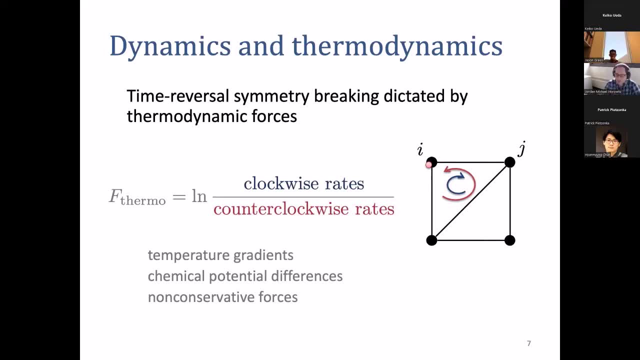 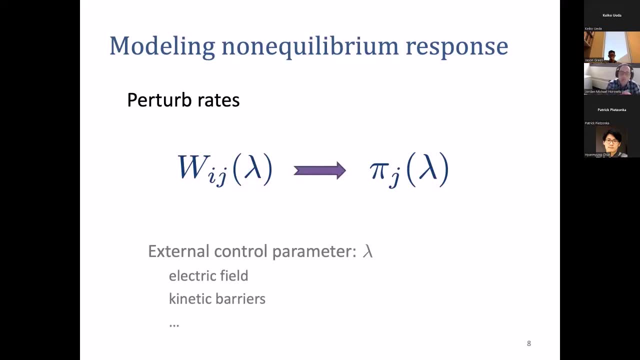 when they appear as a measure of how non-equilibrium the system is. Now within that setup, I'm gonna consider non-equilibrium response And the idea here is now to perturb the system. I'm gonna imagine that my transition rates depend on some sort of external parameter, like we did before. 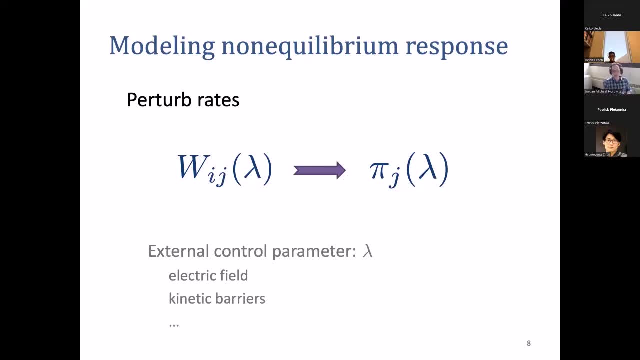 This could be a macroscopic external control field, but as a theorist I can do any game I want, And so I can also imagine connected barriers or varying the charge of an electron, something like that. But whatever it is, if I fix the external parameters and let the system relax, 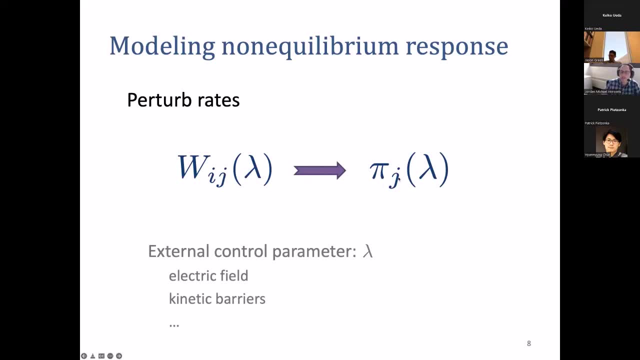 we'll come to some sort of steady state that will depend on that external parameter. And then the question we wanna ask is: how do observables averages of state space variables change when I perturb this external parameter? What are the derivatives of averages? 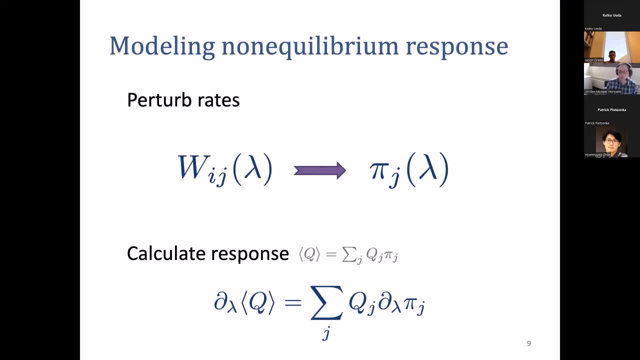 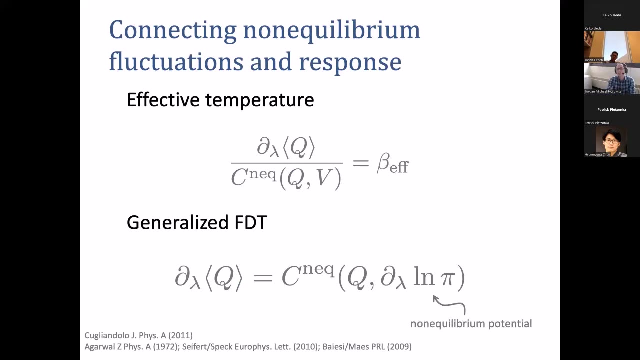 And if I assume that the sort of figuratively but also state-state variables are independent of lambda, then in some sense this question amounts to understanding what is the steady-state response, of just the steady-state distribution, And maybe, if we can get our handle on that, we can say something interesting. So of course this is an 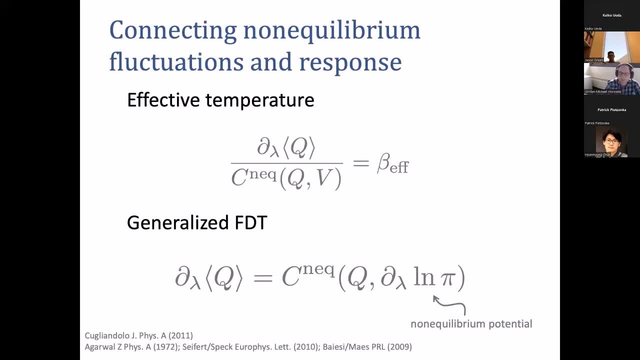 old problem. right, People have been looking at this for a long time. There are many approaches. There are basically two major threads. One approach to kind of rationalize response is to go back and calculate the quantities in the fluctuation-dissipation theorem. the response and now the 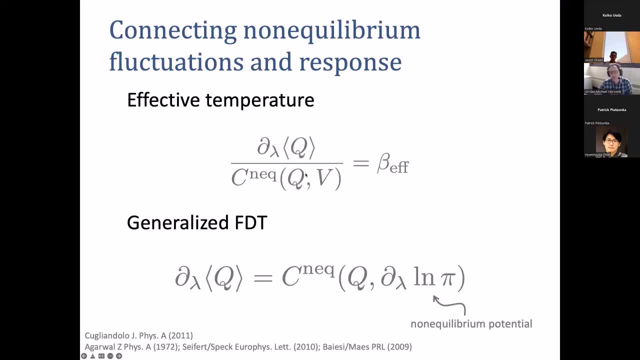 non-equilibrium correlation function. And if I look at this ratio, if the system were at equilibrium, what would appear on the right-hand side would be the inverse temperature. Of course, out of equilibrium it's not a temperature, but people call it an effective temperature. It depends on. 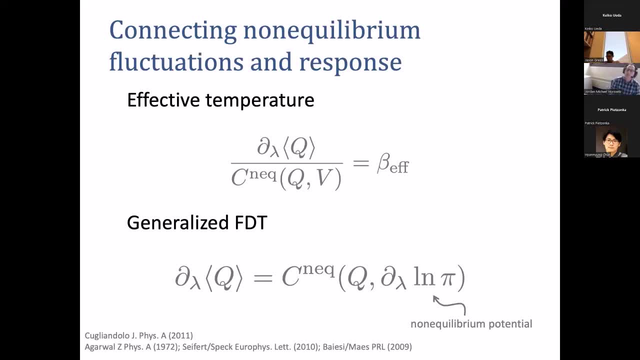 the observables. It depends on many things. Despite it not being a temperature, this is a nice quantity to look at. It's easy to access experimentally, It's fairly easy to calculate in analytical models, So it's a great quantity. 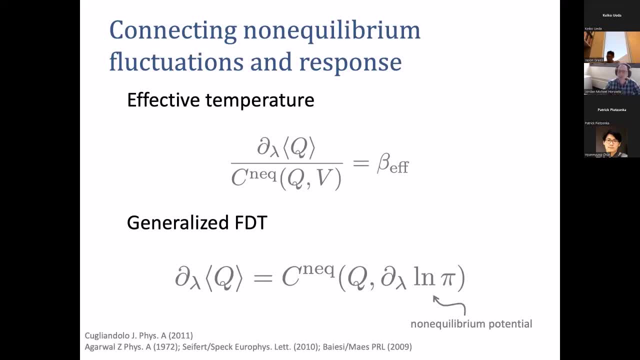 You kind of study models, fit model parameters and try to get a grasp on your system because it includes a number of just interesting properties, Another quantity, another way to do it is to kind of like reestablish the formal structure of the fluctuation-dissipation theorem and write the 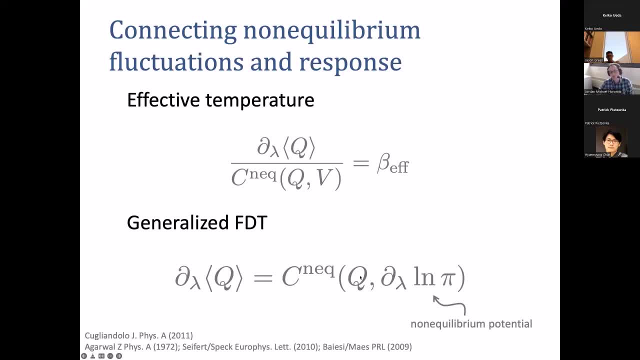 response as now a non-equilibrium correlation function between your observable interest and now some new conjugate coordinate. We've known essentially since the 70s that we can always do this and the conjugate coordinate is the derivative of the log of the steady-state. 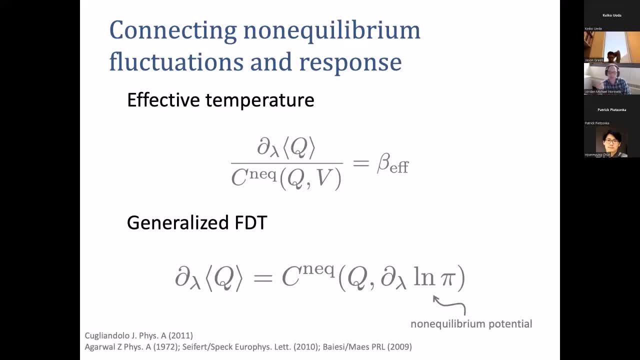 distribution right. This is nice. It's formally exact. It's kind of tricky to use because you have to know the whole steady-state distribution or measure the whole steady-state distribution. That being said, a lot of great work in stochastic thermodynamics have given physical interpretation to this quantity in 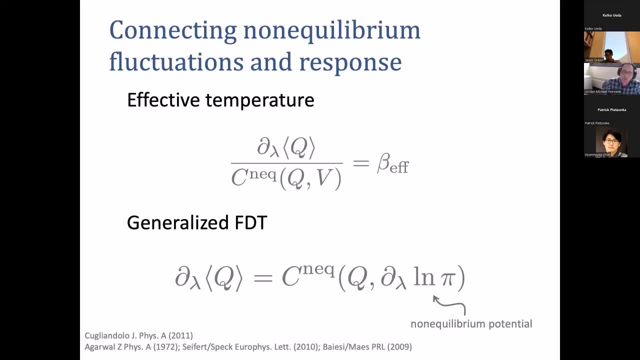 terms of the response of the steady-state entropy production rate as well as, say, the activity or traffic, as we heard before. So this is basically the point: that we enter the top, enter the scope, And our idea here is that instead we're going to try to find out what's going on with the 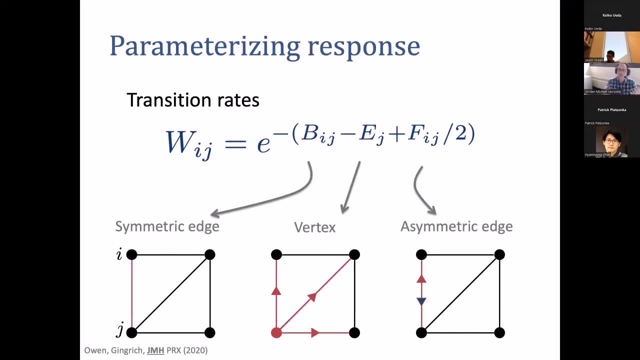 response. So, instead of trying to study the most general kind of response, maybe we can study families of responses and make some analytical progress right? So, motivated by this idea, I'm going to imagine that I can parameterize my transition rate matrix in terms of three. 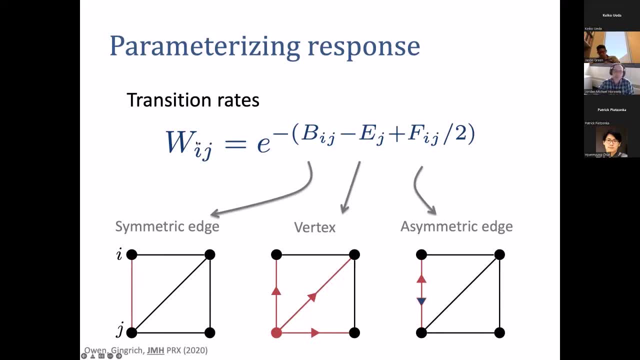 parameters. I'll call b, e and f and imagine that when I change w, I'm only changing some collection of these b's, e's and f's, right? So the b's, they have two indices, so they live on. 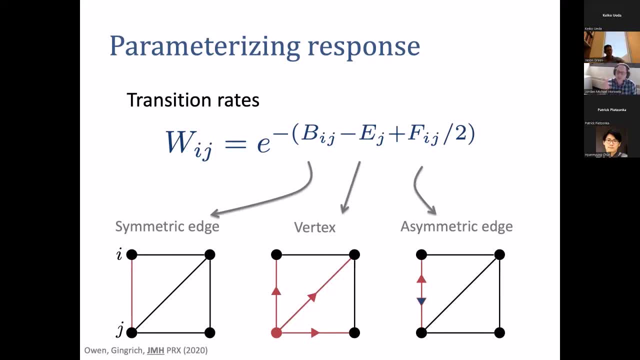 edges and I'm going to assume they're symmetric under the interchange of i and j, so I'll call them symmetric edge parameters. So I'm going to assume they're symmetric under the interchange of i and j, so I'll call them symmetric edge parameters. 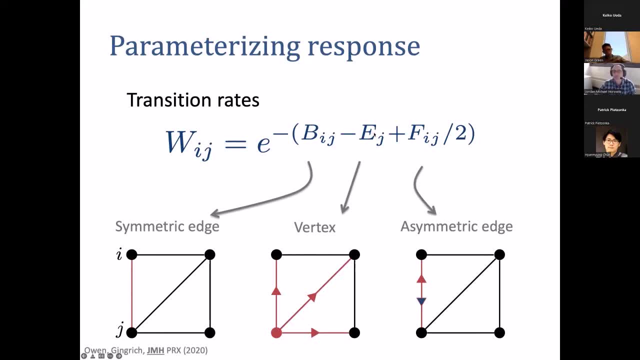 The e's live on vertices, I'll call them vertex parameters. The f's have two indices too, so they also live on edges, and I'll assume that it's anti-symmetric under the interchange of i and j, so I'll call them asymmetric edge parameters, right? 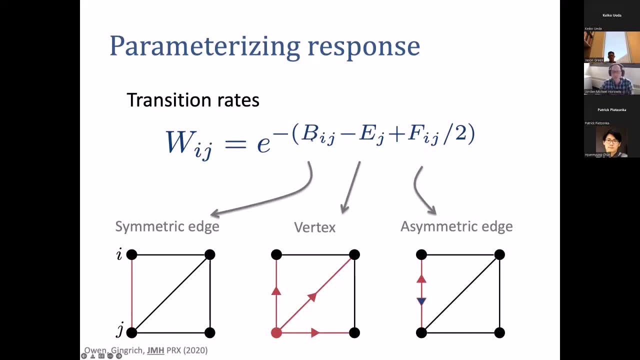 And so if I imagine, if I perturb the system and it amounts to changing one of these b parameters, that's basically like lifting, speeding up and slowing down one edge in this graph. If I vary just the e's, that's like, say, speeding up the exit rate out of a state, and if I say change. 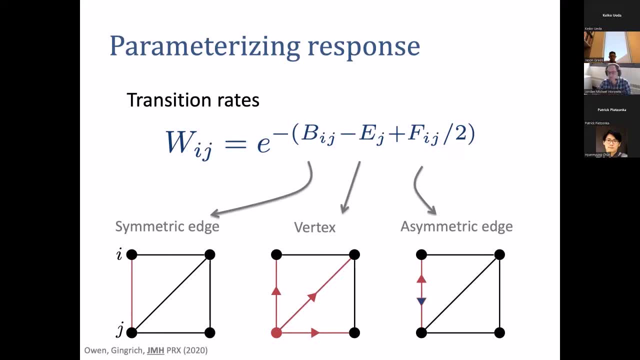 one of these f's, then I'm speeding up one direction and slowing it down right. So the notation here is meant to be kind of suggestive. it's just a mathematical identity. I've just rewritten things. However, it does look a lot like the Arrhenius rate law and that's on. 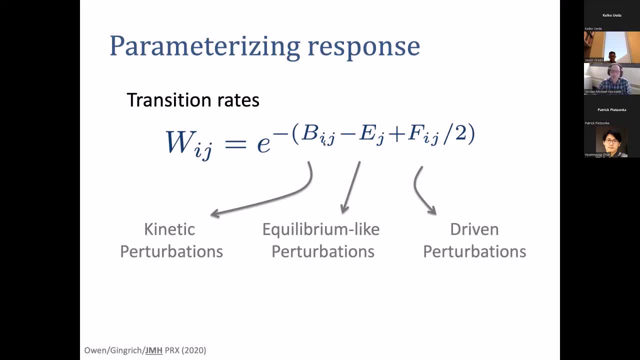 purpose to where the b's are like energy barriers, the e's are like energies and the f's are like asymmetric driving, and this kind of intuition or mapping will be helpful in thinking about the problem. And, in fact, the e's or energies behave very much like equilibrium with respect to 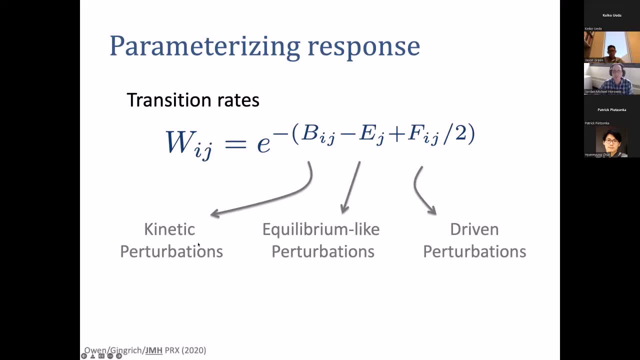 fluctuation, dissipation. The b's are like kinetic perturbations, speeding things up or raising and lowering kinetic barriers, and the f's are like turning on and off external forces. So for each of these families we're able to make concrete predictions. The first one is for these vertex. 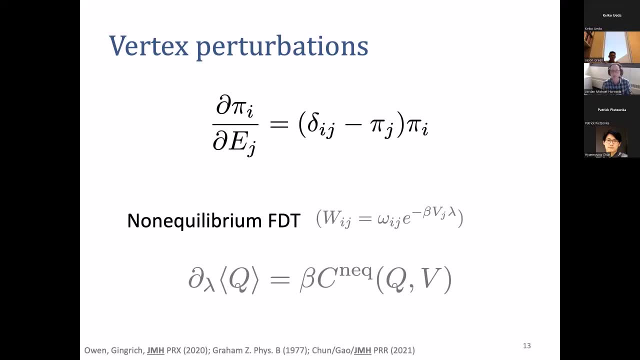 parameters. We can show for any steady state, non-equilibrium or equilibrium, that the response of the steady state of state i to a change in a vertex parameter, state j, has this very simple form in terms of delta functions in the steady state. What's surprising is that there's a lot of 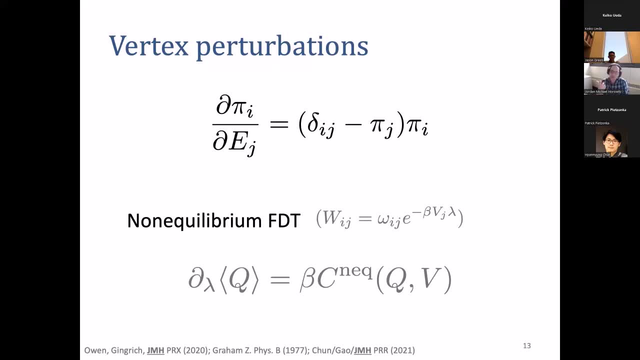 non-equilibrium here. So what's surprising about this prediction is that this is exactly the response you would get if you perturbed an equilibrium Gibbs distribution that just depends on energies. If you perturb that with respect to energies, it's exactly the same. It looks exactly. 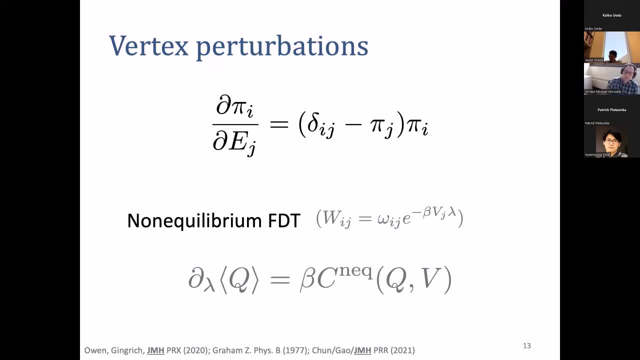 equilibrium-like And in fact we can leverage that by imagining that our transition rate matrix, but we perturb it in such a way that we're only changing these vertex parameters and in which case you can show that the fluctuation dissipation theorem holds identically out of equilibrium. 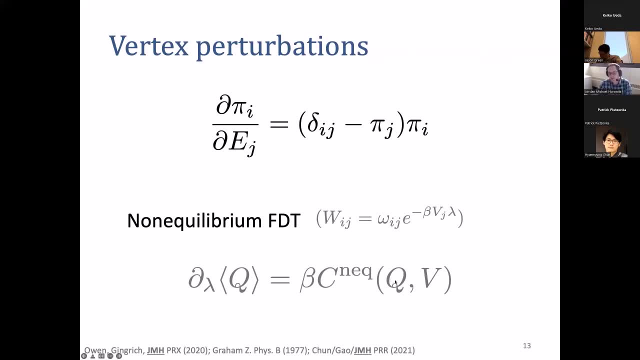 where the response is now the non-equilibrium correlation between the quantity of interest and the original conjugate parameter. Now, we originally showed this for discrete state systems. I have to mention that recent work in the group by Hyun-Yoon Koon has extended this to time. 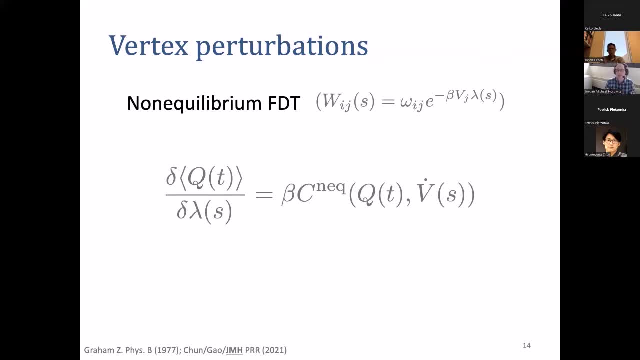 dependent systems, time dependent response, as well as to any kind of Markovian system that evolves under a master equation. It turns out to generalize some very early results from the 70s by Graham, who had done this for the Fokker-Planck equation, And I direct your attention to an article from 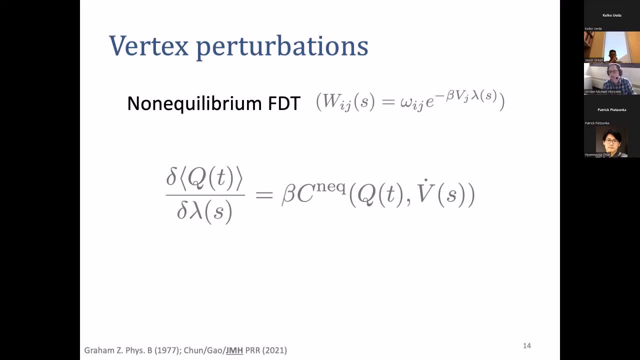 last year where Hyun-Yoon showed that the non-equilibrium, correlation between the non-equilibrium, so that you could use this coupled with the Kubo method to actually calculate Green-Kubo relations for transport in active fluids. But I want to kind of move on from that and talk about the kind of 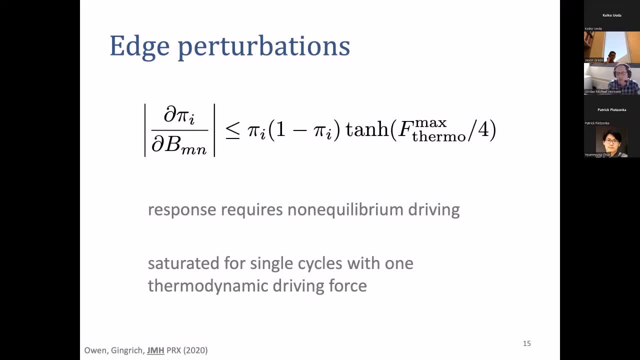 more biochemical type responses. And so our second main prediction is the response of the steady state to one of these barriers or symmetric edge parameters. right, So these symmetric edge parameters or barriers just speed up and slow down reactions. So if you were in equilibrium, 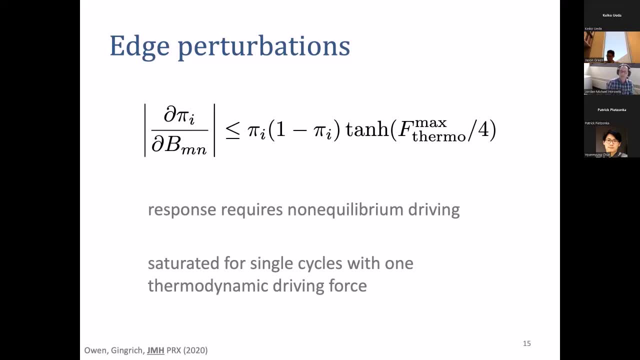 right where the steady state doesn't depend on the kinetics, just the energetics, then you would generate no response. So to get some response you have to go out of equilibrium And in principle you would imagine, the farther you are from equilibrium, the bigger response. 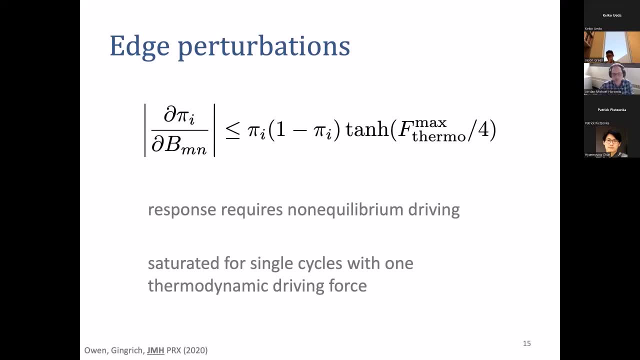 you could get, And so we can show for any non-equilibrium steady state that this response is in fact bounded by pi one minus pi times the hyperbolic tangent of now the maximum thermodynamic driving force in your system right. So the farther you drive the system from equilibrium by turning 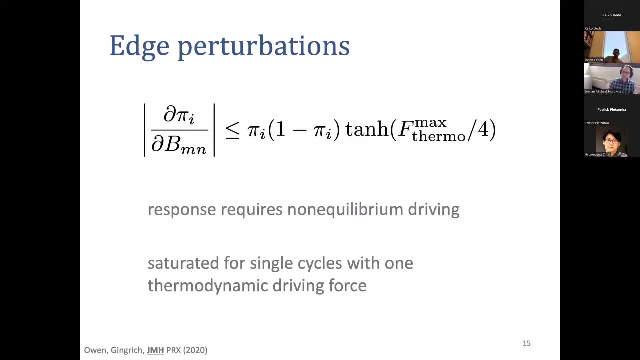 on the external forces, the more response you can get up to some limit. This pi one minus pi in front is the fluctuations in residence time of state i. It's like a Bernoulli random variable, right. So you get this nice little flavor with the fluctuation dissipation theorem. The response: 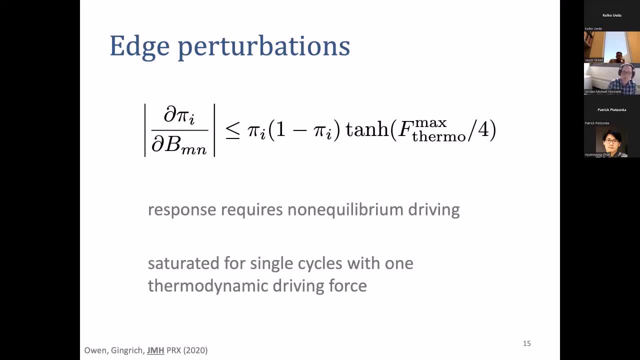 is bounded by fluctuations in thermodynamics. Now, the proof is hard and we don't really understand how to saturate it or how to prove what the saturation is. but I can at least exhibit one example, which is: if your dynamics, your kinetic model, is just a single cycle, it is always possible. 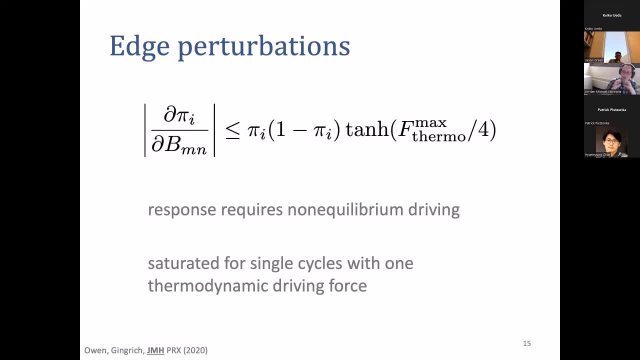 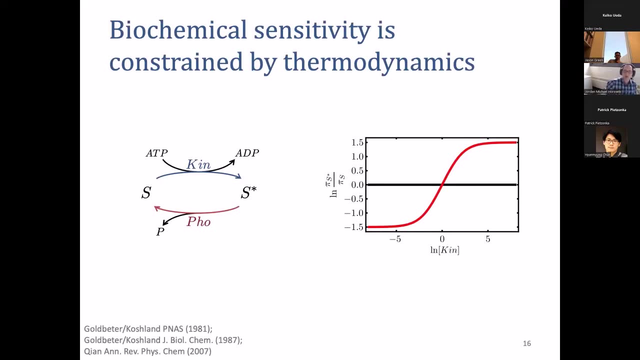 to saturate the inequality. Actually, it's always possible, but you can do it with a single cycle, And so in some sense single cycles are optimal with respect to this response to inequality. So I want to show one quick application to this kind of biochemical response I have in mind here. 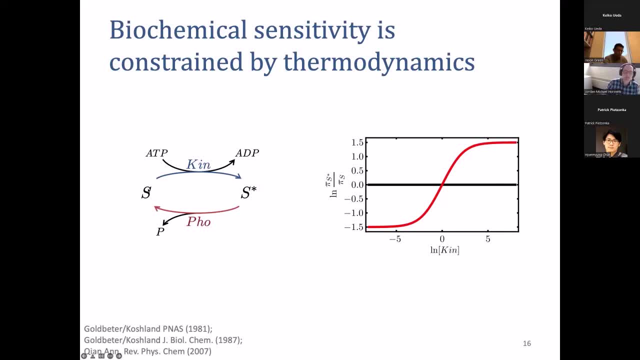 a substrate, a molecule that has two forms, an inactive and active form. So maybe this addition of a phosphate group. So maybe the active form is an enzyme. It goes off and does something else in the cell or in your well-stirred mixture. And if say that active, 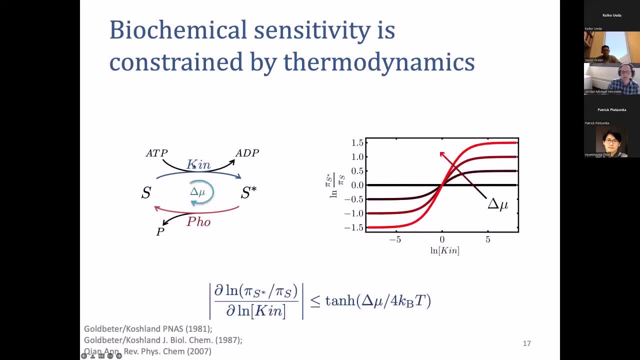 form is the addition of a phosphate, then you might imagine that there's an enzyme like a kinase which adds that phosphate group by pulling it off, an ATP, dropping the residual ADP in a bath, and then the phosphate is later removed by a phosphatase and the phosphate group is dumped. 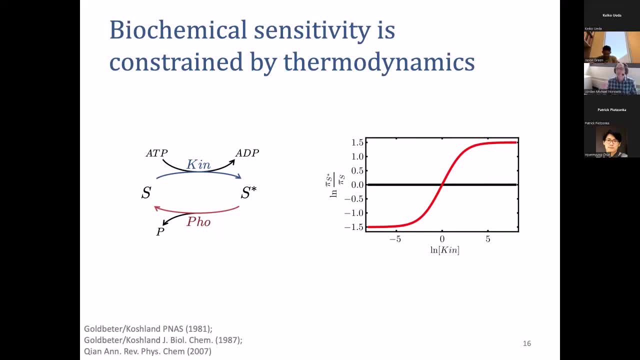 in a bath. So this is a non-equilibrium system continuously consuming ATP and dumping ADP and inorganic phosphate in the bath, And what we'd be interested in is what is the relative likelihood of being in the active or inactive state? that's the vertical axis here, as a function of the kinase? 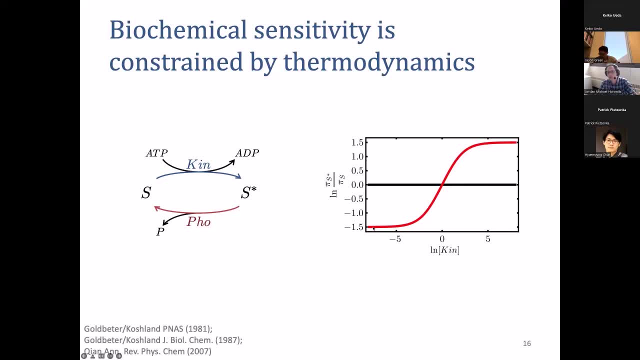 concentration. So you can imagine that as you vary the kinase concentration, you can propagate that signal to the substrate by shifting the bias from inactive to active. And what you can usually show in this model is that as you've increased the chemical potential difference of the ATP with 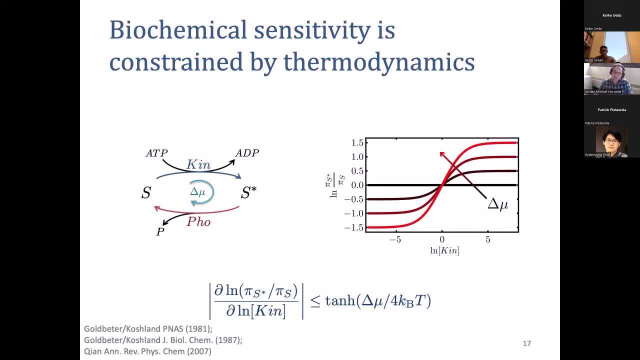 respect to its products. you can make this steeper and steeper and steeper right. And in fact the bound tells us that the log response of the ratio with respect to the kinase is always bounded by the chemical potential. So as you increase the chemical potential, you get a response in the 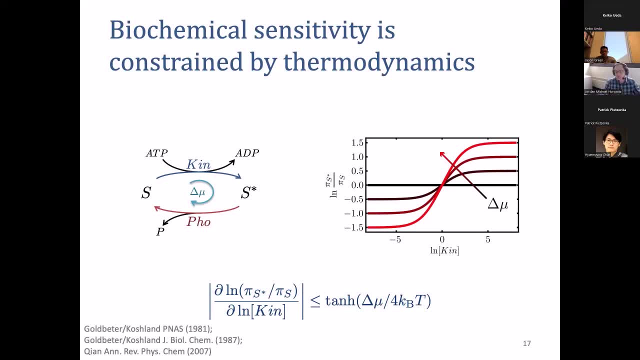 kinase, in this case up to one right. So people in this system- this is called the phosphorylation dephosphorylation cycle. It's a mechanism for zero-order ultrasensitivity And people have known for a long time that this system requires energy. In fact, Goldbetter and Koshland, who originally 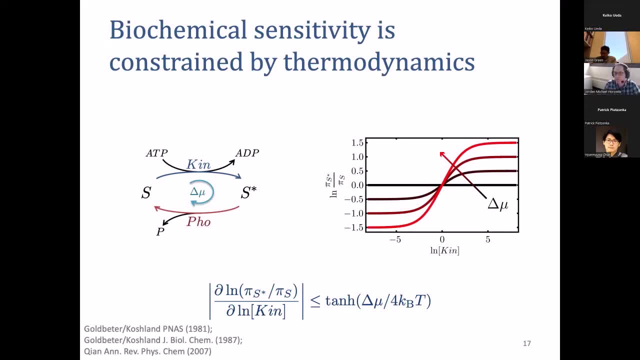 suggested it in a slightly different context, realized it required energy, And this has been studied by Hongshen as well. But what we really have is a rationalization of that. We can say what we can do without really making a lot of detailed modeling assumptions. 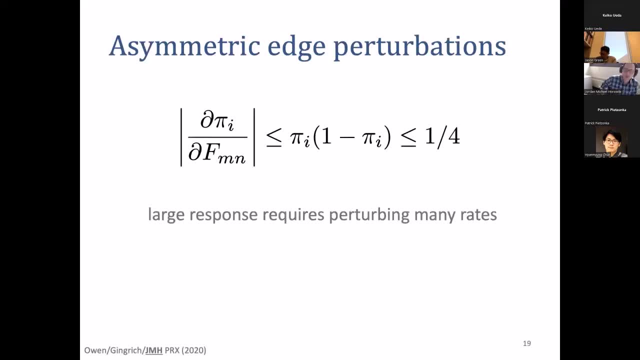 We can also say something about the response to the force. That's always bounded by one quarter. In fact all the bounds are bounded by a quarter. So if you only perturb one edge in your graph, there's a limit to the response you can get. So in principle, if you want to get very big response, 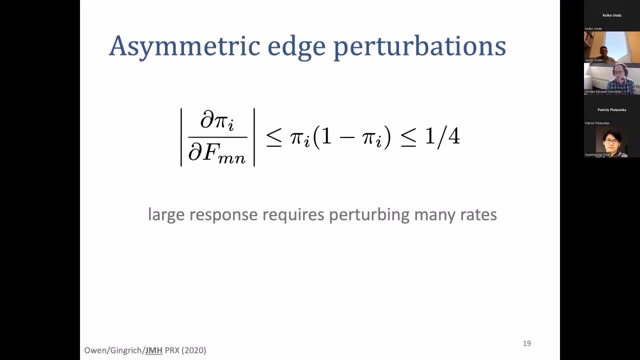 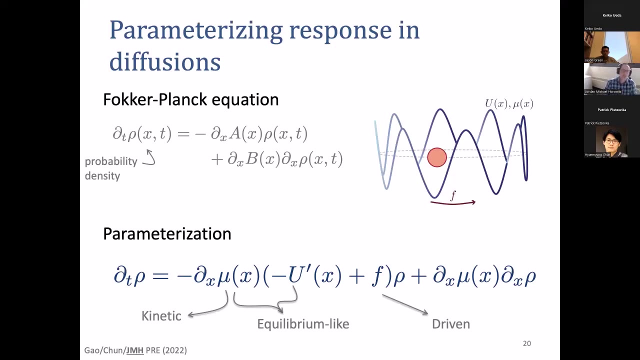 you have to perturb many edges And it seems to grow linearly. Well, that's not true, Sorry. You have to perturb many edges And the more you do in principle, the more response you can get. Okay, So with the last couple of minutes I want to talk about some recent stuff. 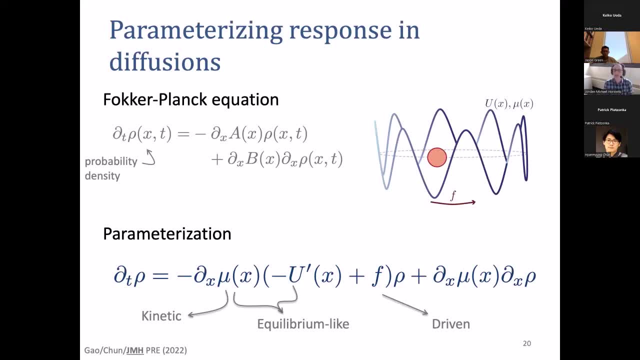 And so you might ask what happens. if we look at a diffusion process, It seems like a natural question to ask, And so I'm going to talk about how we can repeat this program in the context of a one-dimensional diffusion, only in 1D, because that's all we actually understand at the moment. 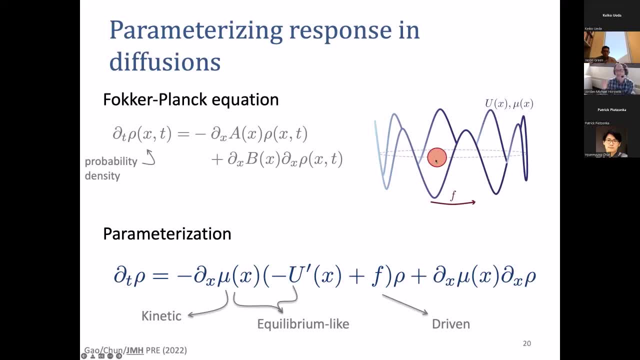 So for a particular one-dimensional diffusion process, say like a particle on a ring, the evolution of the probability density is given by the Fokker-Planck equation. There are two parameters. The probability density is given by the Fokker-Planck equation. The probability density is: 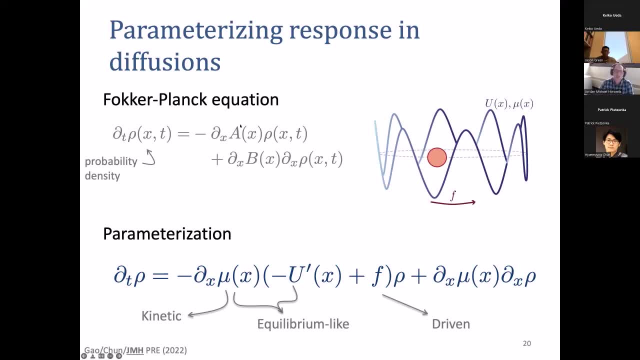 called the Fokker-Planck equation. There are two parameters that enter into the response. There is the drift term a, which I'll call a, and the diffusion term, which I'll call b. And now the question and response is if I vary some actual parameter that varies, the a term or the. 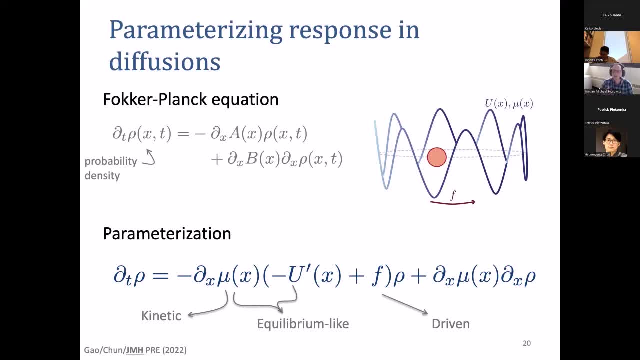 b term, how much response can I get? And so, motivated by the discrete case, in fact, by discretizing the diffusion process and studying the discrete case in this context, we came up with the following parameterization of the response into three functions, which are called mu. 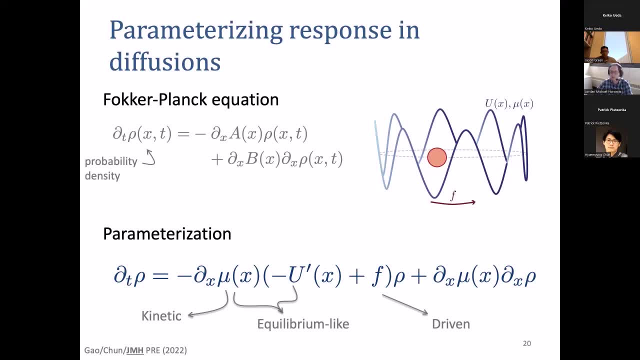 u and f, which are very much motivated by the mobility, energy and force of a single driven particle. So you can rewrite the Fokker-Planck equation: as the derivative You have your mobility, some energy and a force. This is just re-parameterizing A and B, just 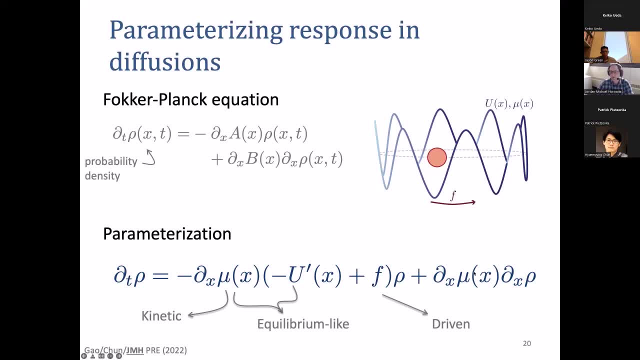 mathematically and as well as the mobility inside the noise term right. So you can think of these parameters like a single ideal gap, single colloidal particle on a ring, some external force with energy and spatially dependent energy and mobility. And now you can ask: 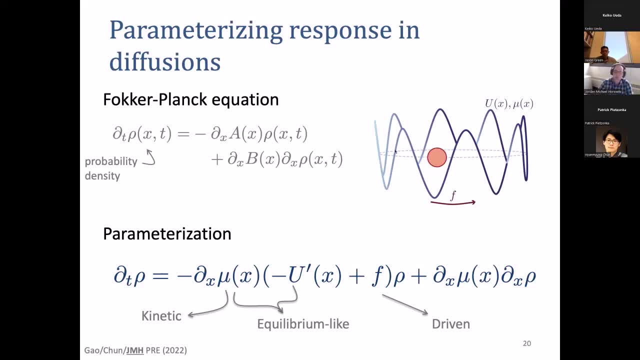 what is the kinetic perturbation? What is the equilibrium-like perturbation? Well varying, these mobilities ends up being just like the kinetic perturbations of raising and lowering energy barriers. What's perhaps more surprising is that the equilibrium response, if you want. 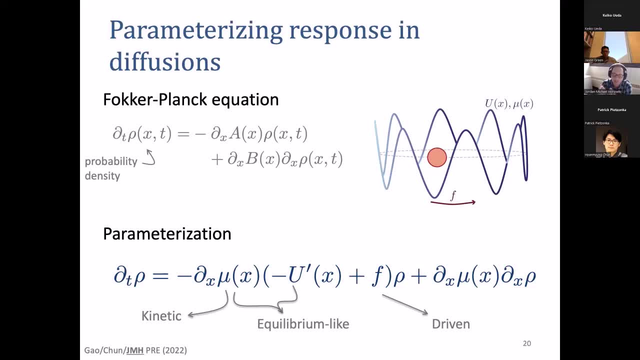 to generate or do a perturbation that results in an FTT. identically, you have to perturb the energies and the mobilities in unison, right. This is why, when you perturb the energy alone out of equilibrium, you don't get a simple answer And in this case, the driven for driven response. 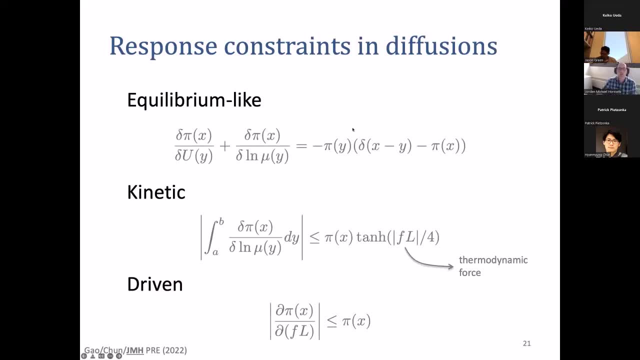 is captured by the non-conservative force. So in particular, we have a number of equalities, inequalities, that the equilibrium-like response- if I perturb the energy and mobility in a particular point has an equilibrium-like structure. The kinetic perturbations, where 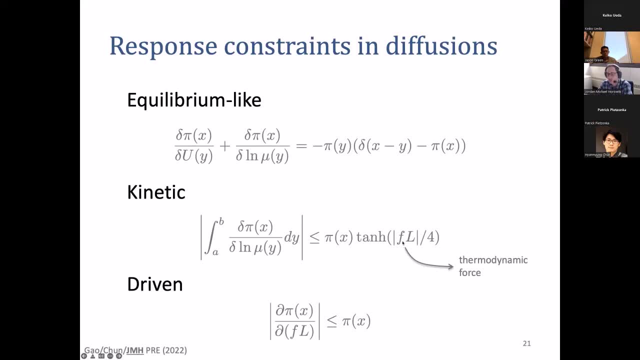 I perturb, the mobility is bounded by the hyperbolic tangent of now the thermodynamic driving force of this system. the force times the length around the circle And in general, response is always bounded. The mathematical results here are slightly different and have some subtleties dealing with the fact that you're dealing with a probability. 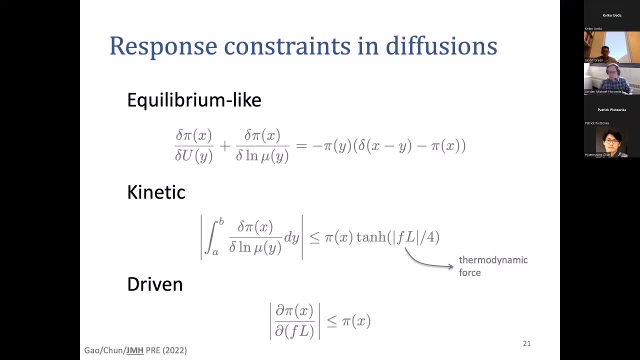 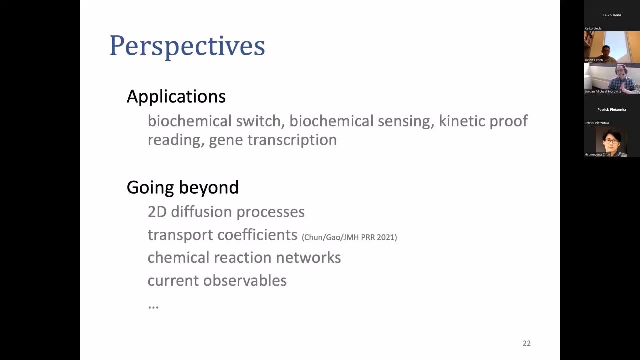 density instead of a probability distribution. But at least for 1D it seems to work. We're still working on 2D, So with that I'll conclude. I talked about some bounds and equalities for non-equilibrium response. It was the fundamental theory section, so I shied away from applications. 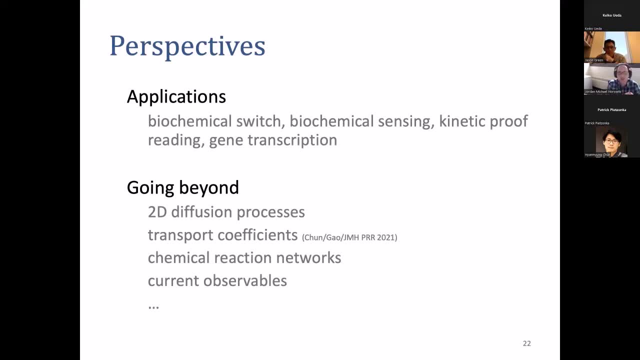 as much as I could, But we have looked at using these to understand response in biochemical switches, like we looked at some simple motifs like biochemical sensing, kinetic proofreading, gene transcription, simple networks, And we're also looking in different directions. Chi, who did the 1D diffusion process. 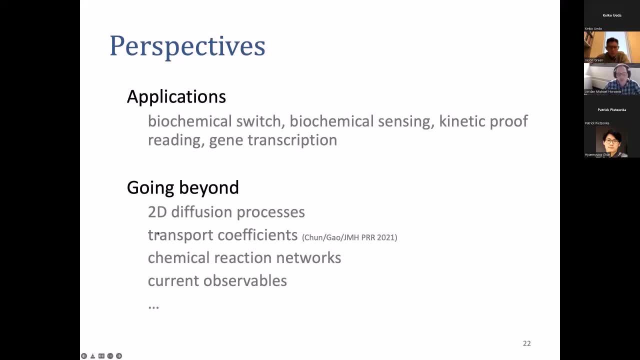 is working on 2D processes. I mentioned this work by Hyun Myung on transport coefficients, And now we're also trying to think about how does this have something to do with chemical reaction networks, which are more biochemical relevance, as well as extending them to other